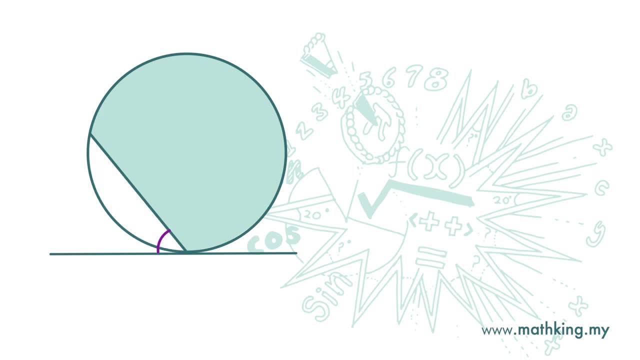 here Now. this angle is equal to the angle. here in the major segment, which we will call alternate segment, The angle can be this or this or this. All these angles are equal because they are subtended by the same arc. Similarly for this angle that is subtended by the tangent and this chord. 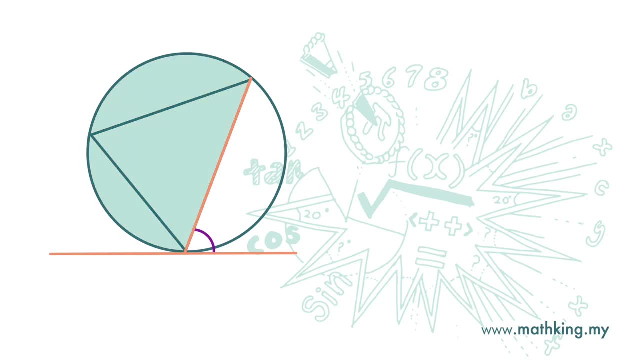 the alternate segment is this: and this angle is equal to this angle in the alternate segment. Now, why is that? so We can draw two lines from the vertices here? We can draw two lines from the vertices here. Now, why is that? so We can draw two lines from the vertices here? 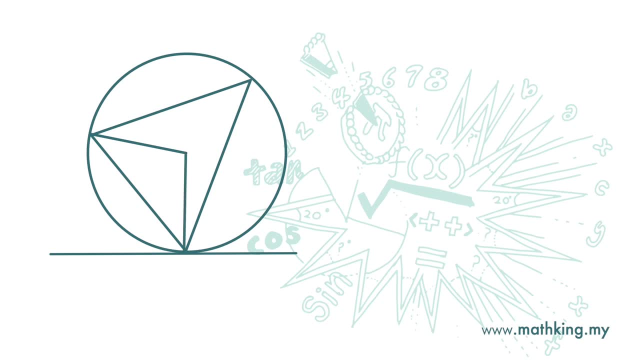 here to the center. Now angle X and angle A, when added up, is 90 degrees, because we know that a tangent makes a 90 degrees angle with the radius of a circle at the point of tangency. Next we will draw a perpendicular bisector from center O, So it is 90 degrees here. 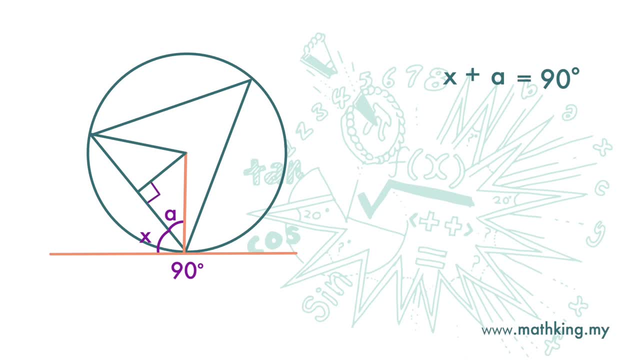 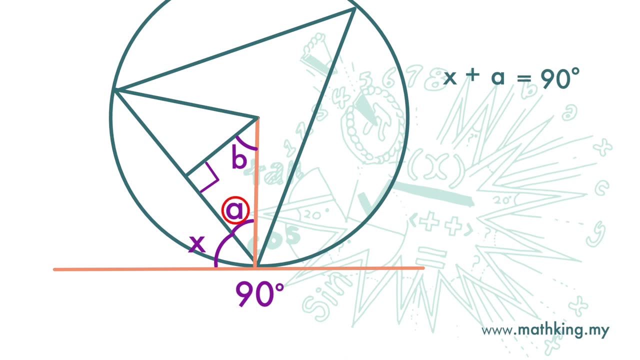 Now we call this angle here B. Note that angle A and angle B also add up to 90 degrees, because in this triangle A plus B plus 90 degrees give us 180 degrees. So A plus B is 90 degrees. Then we 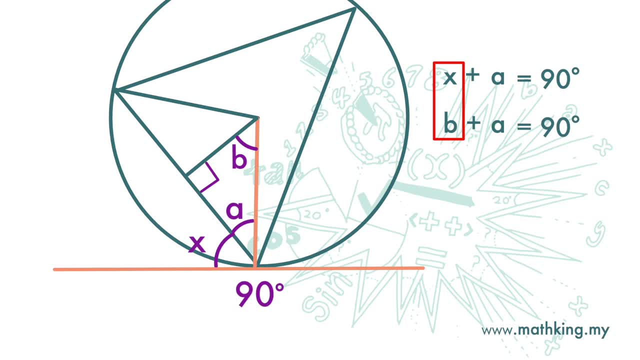 can see that B equals X, So we are going to denote this angle here as X. Then this whole angle will be 2X. Now this angle at the center is subtended by this arc. This same arc also subtends an angle at the